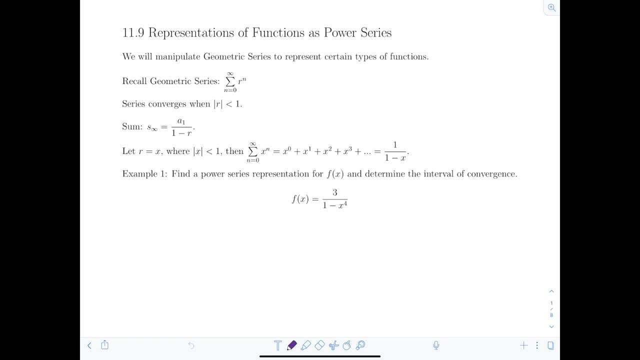 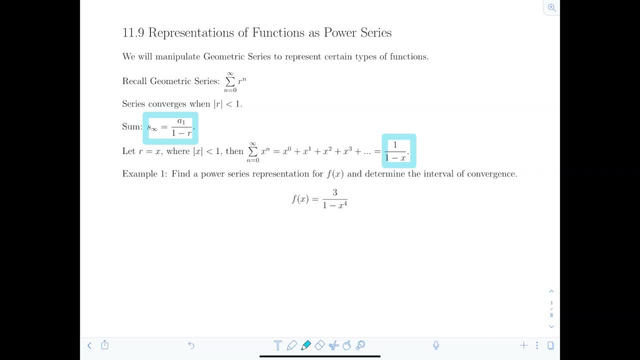 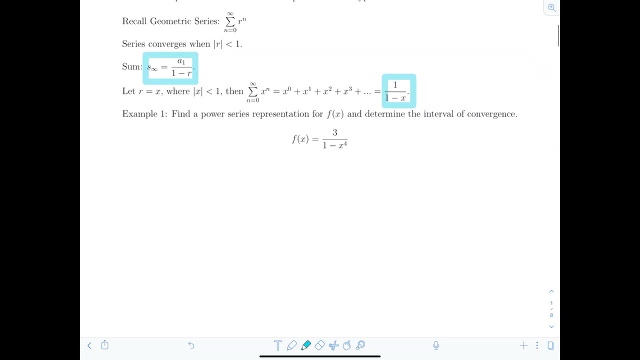 of r to the m of r to the m of r, r to the m of x. here There's a 3 in the numerator. I want a 1 in the numerator, So I'm just going to write it out in the front And then I have 1 over, 1 minus, And let's put some parentheses here. That. 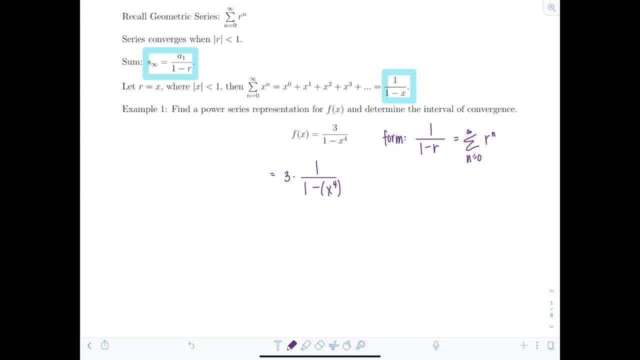 way we can really focus on that. x to the fourth. Now notice, I basically already have my desired form right. x to the fourth is going to be r, And then the only difference is now I have to multiply my sum or my series by 3.. But that's not a problem, So let's go ahead and do that in the 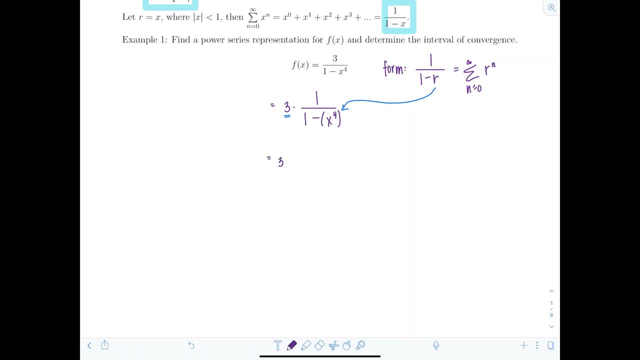 next step, I'll keep 3 outside the sum And then we'll write summation: n equals 0 to infinity And r is x to the fourth. So I have x to the fourth to the n. Okay, And then from here. 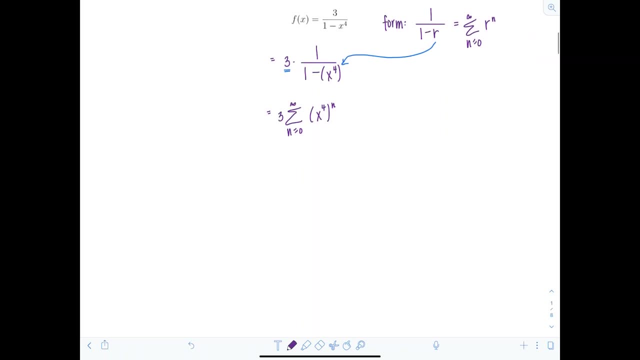 you just want to simplify your series as much as possible. So this means f of x, which is equal to 3 over 1 minus x to the fourth, I can write as: the sum n equals 0 to infinity, of 3x to the 4n. Okay, Now this power series representation. 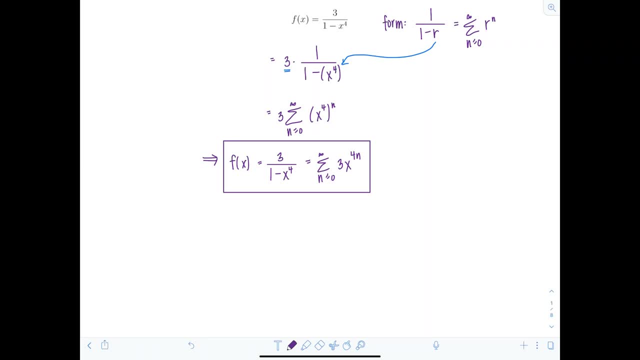 is only valid for certain values of x that fall within the interval of convergence. How do I find the interval of convergence? Well, when working with power series, all you need to do is recall the fact that the absolute value of r needs to be strictly less. 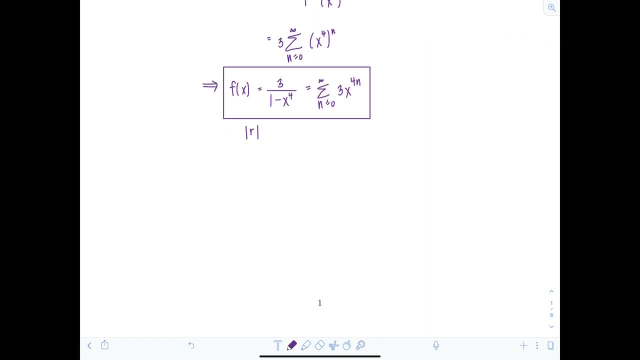 than 1.. So you don't have to apply a test, like you did in previous circumstances, When finding the interval of convergence. So, absolute value of r, which in this case would be absolute value of x to the fourth, we require that it be strictly less than 1.. Well, x to the fourth is: 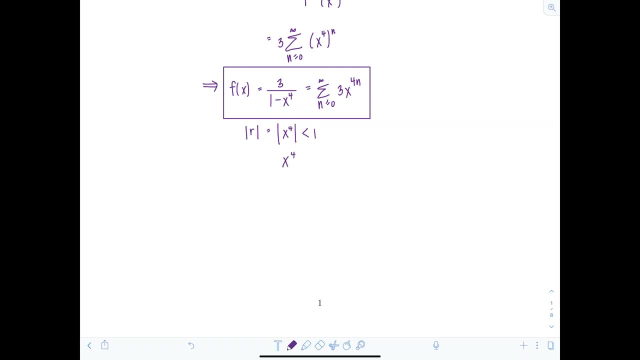 always positive. So I don't need absolute value. I just need to make sure that x to the fourth is less than 1. And that will be satisfied so long as x's are strictly between 1 and negative 1.. So I know my interval of convergence is the interval from negative 1 to 1.. I don't need to. 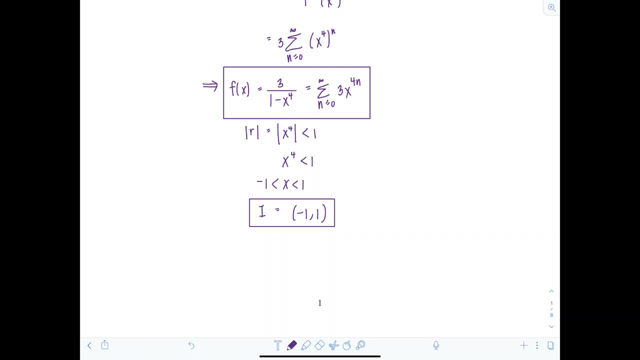 find points, because I know for a fact: the geometric series will diverge if r is equal to positive or negative 1. So all I need to do is just solve for the interval. that works, and that's it All. right, Let's move on to another example. So find a power series representation for f of x. 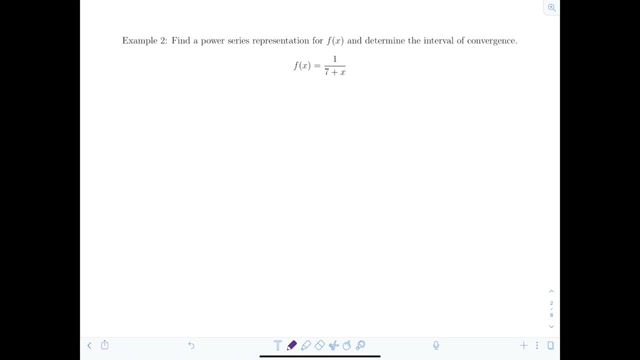 and determine its interval of convergence. So same deal as before. Remember, I want to try to write it in the form 1 over x to the fourth. So I'm going to write it in the form 1 over x to the fourth. 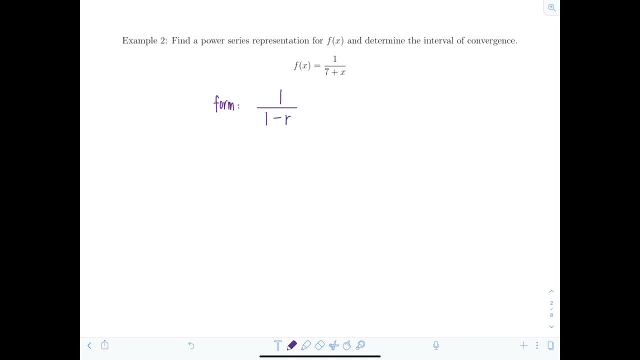 1 over 1 minus r. All right. Well, the only issue that's maybe glaring at us right now is the fact that this is a 7 and not a 1. So let's get started with fixing that. Now I can factor that 7 out of. 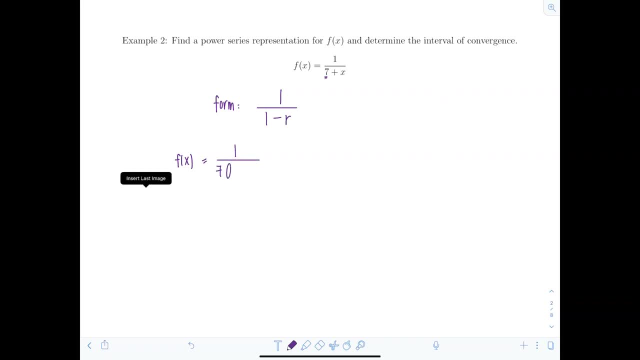 the denominator. And now I'm going to be left with 1 plus x over 7.. OK, So things are looking a little bit better. And then, remember, I need 1 minus r. So this is the denominator. So this is 7 times 1 minus negative x over 7.. And then now I've. 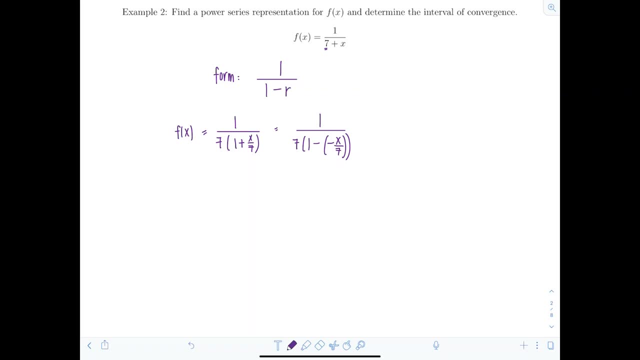 rewritten f of x so that I can clearly identify what r would be. So I'm going to have 1 seventh sitting outside the sum We have. 1 seventh times the sum n equals 0 to infinity. And now I'm going to have negative x over 7 raised to the n. OK, 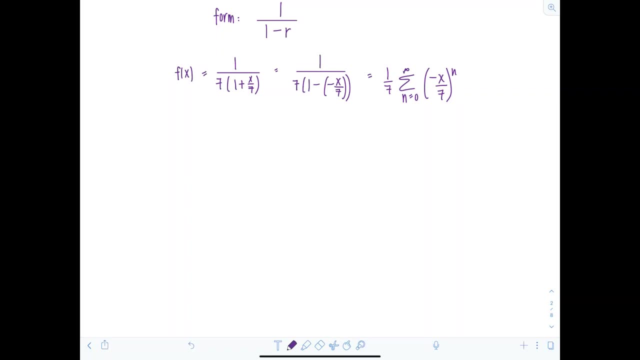 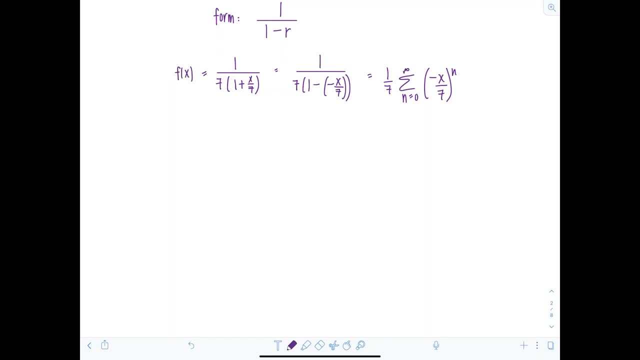 you have an alternating series, So you want to separate that. That way it's very clear. And then also that 1 seventh, I could bring it inside the sum, So I have the sum n equals 0 to infinity. I want to write this as negative: 1 to the n times x to the n over 7. It's going. 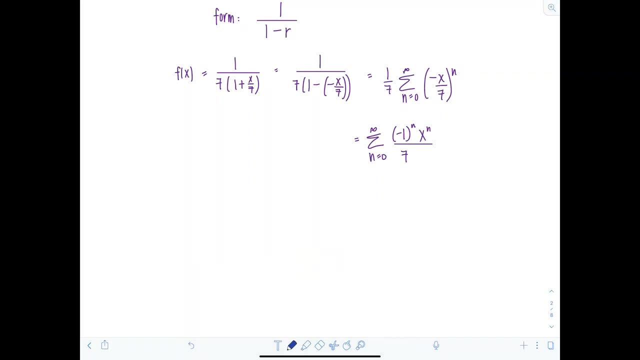 to be raised to the n, but then I'm going to bring in this 7 as well, So now I'm going to have my exponents going to be n plus 1.. OK, So there's our power series representation for f of x. Now I need to find the interval of convergence. 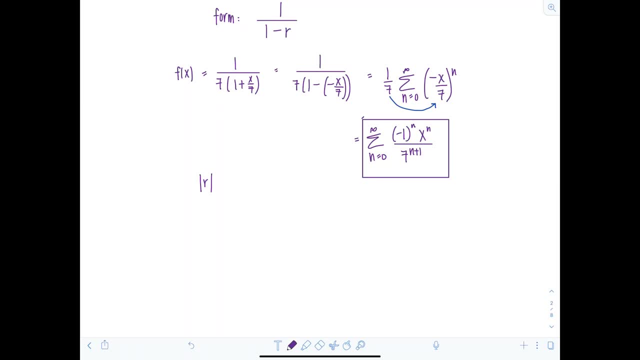 Well, I need to impose that the absolute value of r be less than 1.. Where's r? Don't look for it in the most cleaned up version of your sum. The easiest place to find r is right here, before you out your power series. So this is going to be the absolute value of negative x over 7 has to be less. 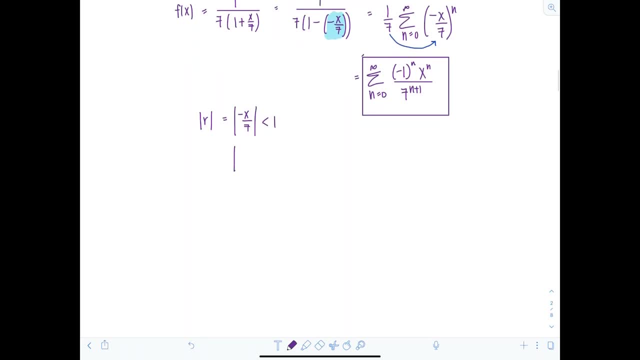 than 1, okay, So if I take the absolute value, I'm just going to have absolute value of x over 7, the negative goes away is less than 1, which would mean the absolute value of x multiplying both sides by 7 would have to be less than 7, strictly less. So the interval of convergence. 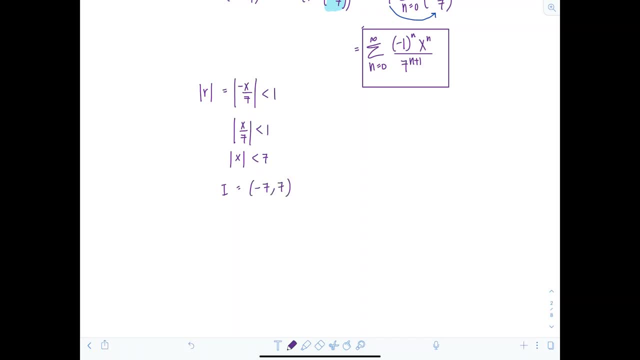 is going to be from negative 7 to 7, not including the endpoints. All right, let's move on. maybe something a little fancier. So same directions find a power. series representation determine the interval of convergence. So I'll remind you. 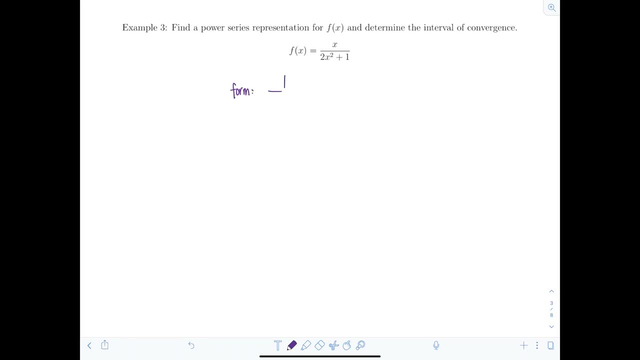 the form that we want to mirror or use as our model is 1 over 1 minus r, because then I can write it as 1 over 1 minus r. So I'm going to write it as 1 over 1 minus r because then I can. 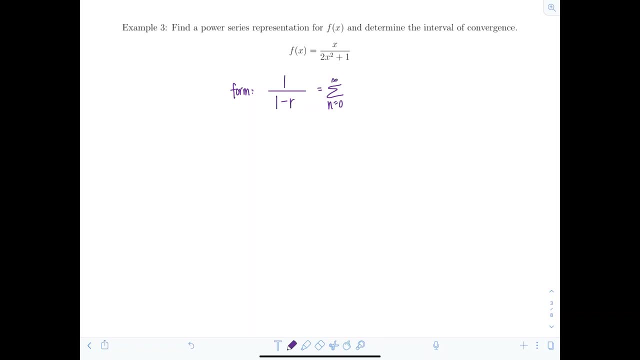 write it as 1 over 1 minus r, because then I can write it as 1 over 1 minus r, because then I can write it as the sum n equals 0 to infinity of r to the n. Okay, well, let's see here: there's an extra x in the numerator. it's not a 1, so I can fix that. 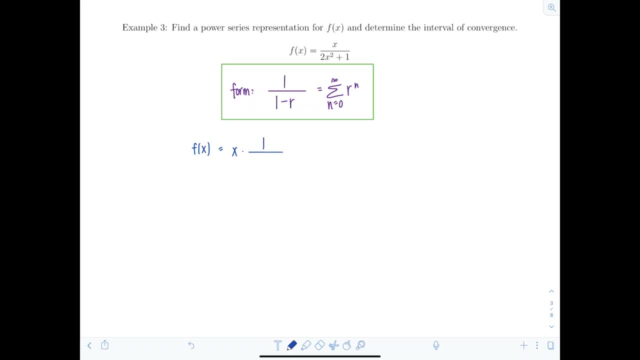 no big deal, x times 1 over. and then, just to help us visualize, I'm going to interchange the order of addition in the denominator. not a big deal, but it'll help us. So now I have 1 plus 2x squared. in the denominator, and then I'm going to write it as the sum n equals 0 to infinity, of r to the n. Okay, well, let's see here there's an extra x in the denominator, and then we're pretty much done. 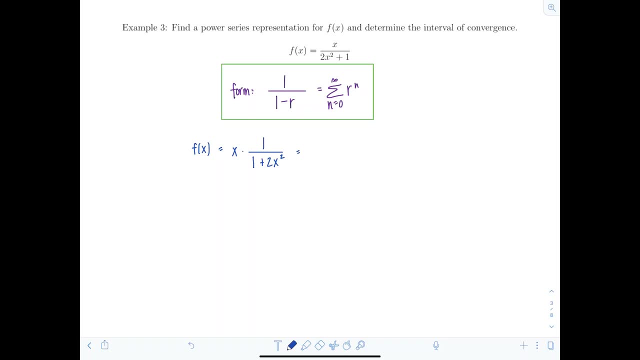 because I can just easily rewrite that addition as subtraction if I change 2x squared to negative. So I have x times 1 over 1 minus negative 2x squared, and then we can see here this is going to be our r, So I can write this as: x times the sum n equals 0 to infinity of negative 2x squared. 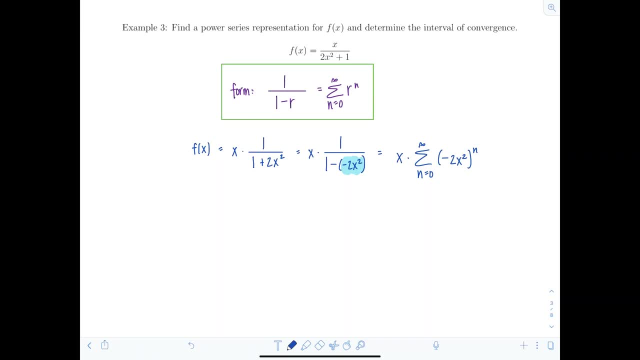 to the n. Okay, so that means my function f of x, which was originally x over 2x squared plus 1, I can write that as the sum n equals 0 to infinity. Now notice, here I have this negative. 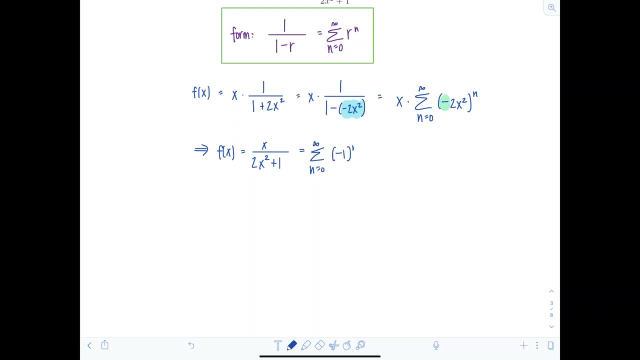 so I want to always write that separately. So I have negative 1 to the n, then I'm going to have the n distribute to the 2x squared to the n. So I'm going to have the x to the 2n, but then, don't forget, there was this x sitting outside. 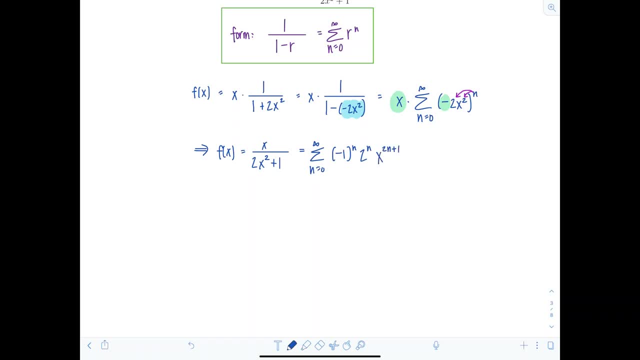 so I'm going to be left with x to the 2n plus 1.. All right, and that's my completely simplified form. Oh, no, Beautiful Okay, and then. now it's time to find the interval of convergence. So, remember, we require that the absolute value of r, which do you remember where's 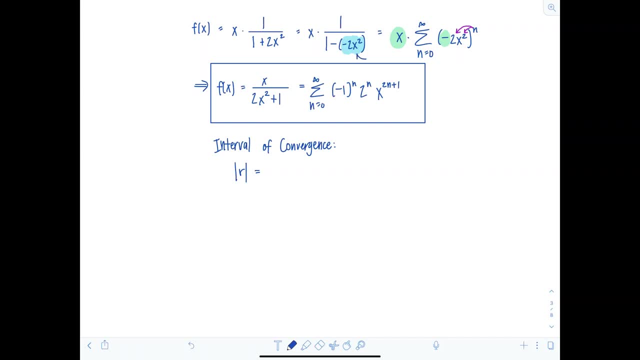 the easiest place to go find r. It's right here before we wrote our Power Series out. So the absolute value of r would be the absolute value of negative 2x squared. that needs to be strictly less than one. I can rewrite this as the absolute value of negative 2 times the absolute value of x squared. x to the 9x squared has to be less than 1.. I can rewrite that for randomDAO. I can rewrite this as negative 2 times the absolute value of x squared has to be less than 1.. So this: if I find r- 0 until r- تعocracy, I have 2, that means it's the absolute value of. I found at y, because I try to add this and multiply this. 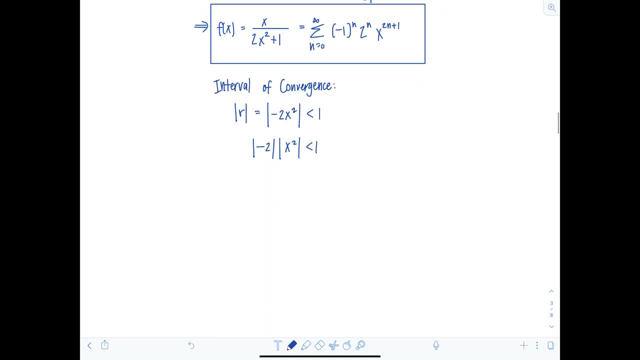 less than 1.. Well, the absolute value of negative 2 is just 2.. I could divide both sides by it and then x squared is always positive, so I can just have x squared needs to be less than 1 half. 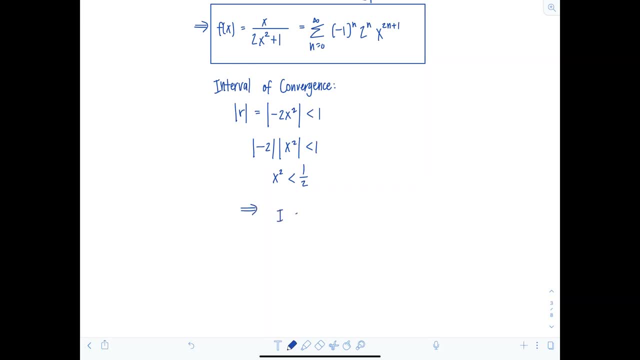 which means that my interval of convergence is from negative- 1 over rad 2- to 1 over rad 2.. All right. Example 4, express the function as a sum of a power series by first using partial fractions, then determine the interval of convergence. So I'll let you make sure you. 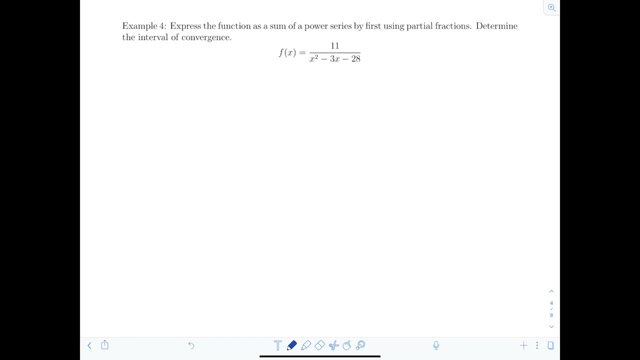 can remember how to do partial fraction decomposition. Remember, you're going to start off by factoring the denominator for f of x, so I can write it as 11 over rad 2.. So I'm going to start off by factoring the denominator for f of x. 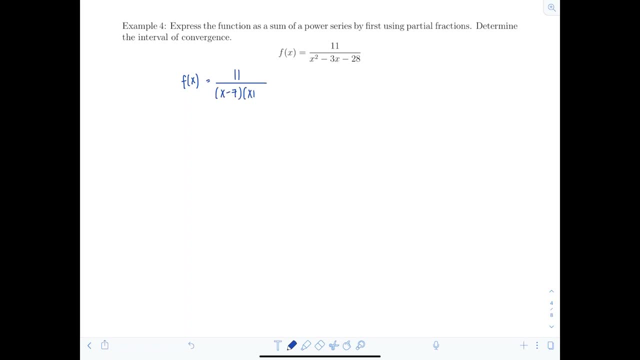 so I can write it as 11 over rad 2.. So I'm going to start off by factoring the denominator for f of x over x minus 7 times x plus 4.. And then you should end up with 1 over x minus 7, plus negative 1. 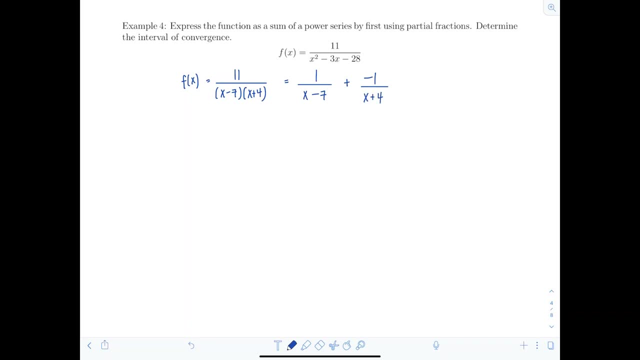 over x plus 4.. All right, So this means I'm going to find a power series for 1 over x minus 7 and negative 1 over x plus 4, and I'm going to end up adding these together in order to represent f of. 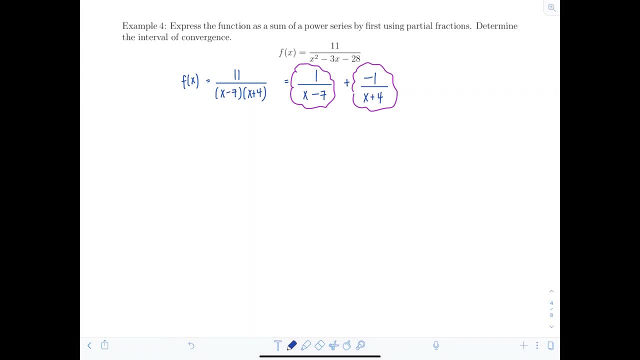 x plus 4.. So, to start off, for 1 over x minus 7,, I really want to reverse the order of subtraction in the denominator, so I'm going to write this as negative: 1 over 7 minus x. And then for the 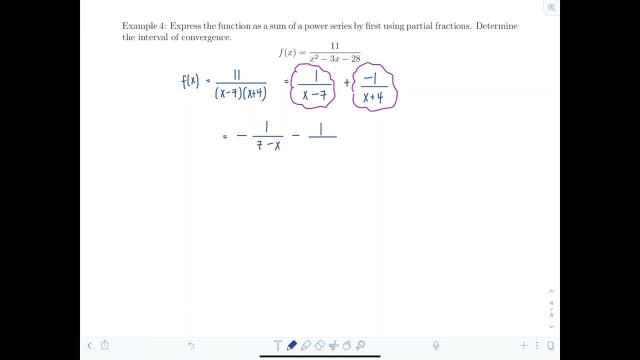 next term. I'll just leave that negative outside and then I'll have 1 over. let's switch that 4 in the x, so we have 4 plus x in the denominator instead, And then now we've been in this situation. 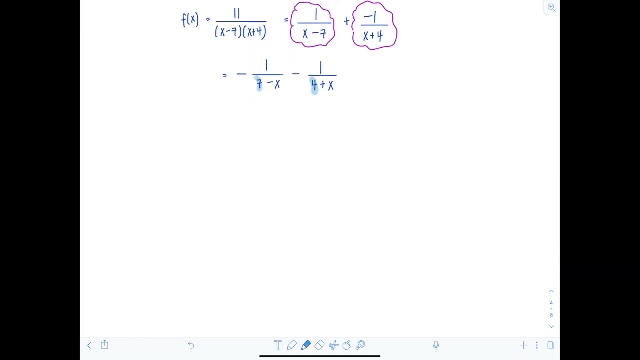 before. so I can factor out the 7 from the denominator and factor out the 4 to make those both 1s. So now I'm going to have negative 1 seventh times 1 over. this is going to be 1 minus x over 7,. 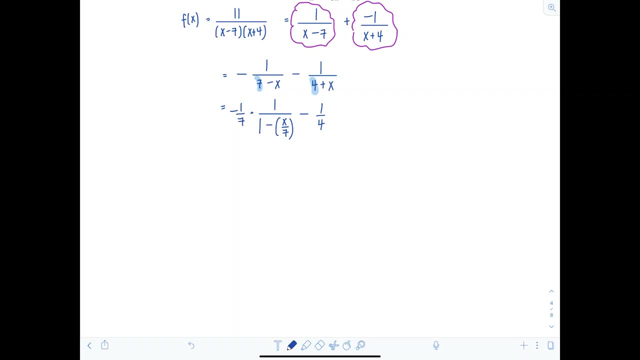 minus. and then now I have 1 fourth times 1 over 1, minus negative x over 4.. All right, Don't forget to switch the addition to subtraction. and then now I have a negative x over 4.. Okay, So let's start writing this out. 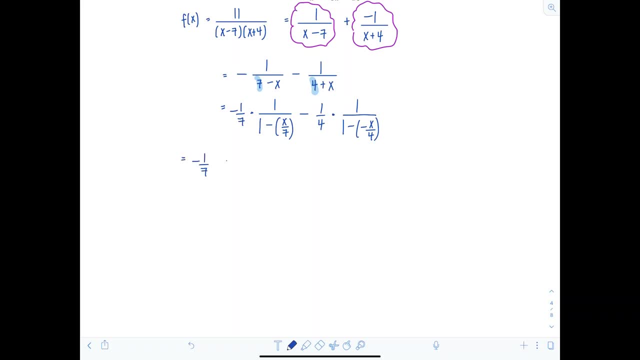 So here's my equation below and here's an總 to Jacques. So here's the solution. so now, given the relationships, choose, because even if you click with, you'll also get the same. c верх, go close to the center and off to the center. 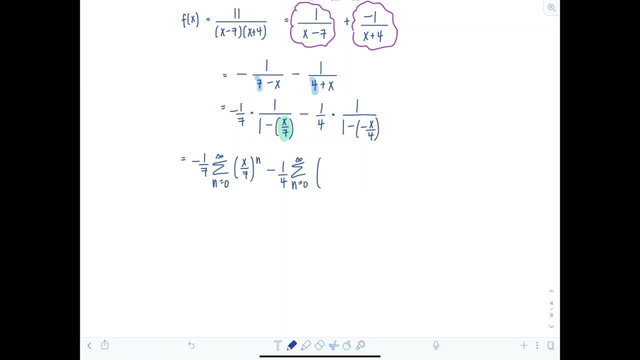 Right. So what does that mean? So this is negative: 1 over 7 times 1 over 2.. Now, if we're required here, then that's going to have 1 diminutive distance, which is also the root. All right, 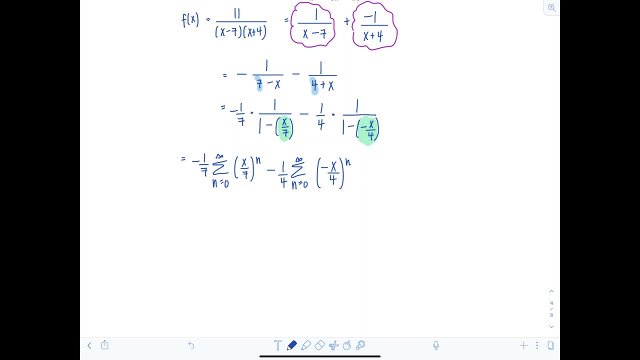 All right, 4 raised to the nth power. Okay, so let's see how far can we take this when we're cleaning up. Well, one thing I notice is I could bring this 7 inside, and I can also bring this 4 inside the sum. 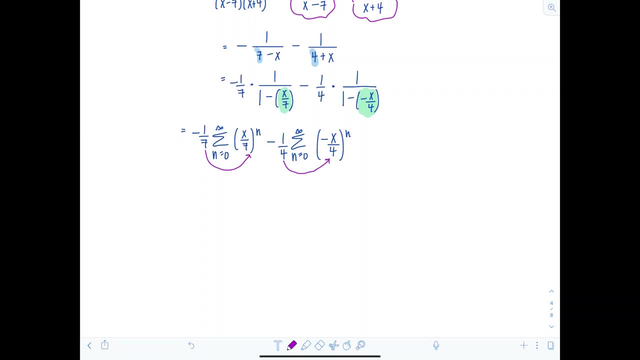 and just add one to the exponent. So we're going to have here- let's leave that negative outside- and then we have the sum n equals 0 to infinity. I'm going to distribute numerator and denominator to the nth power, so we'll have x to the n over 7 to the n plus 1. now minus, the sum n equals 0 to. 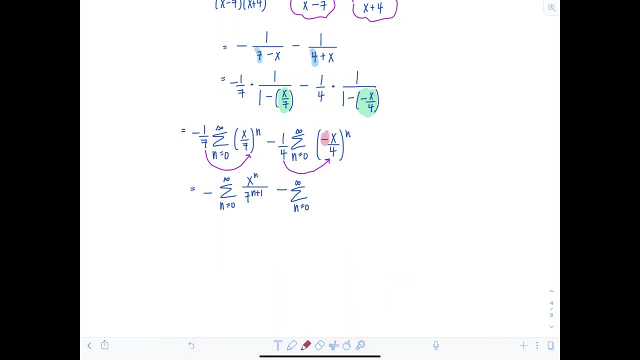 infinity. Now notice, because we have this negative here, that one's going to be an alternating series, so I'm going to have negative 1 to the n x, to the n over, 4 to the n plus 1.. Okay, now notice both of these. the indices started. 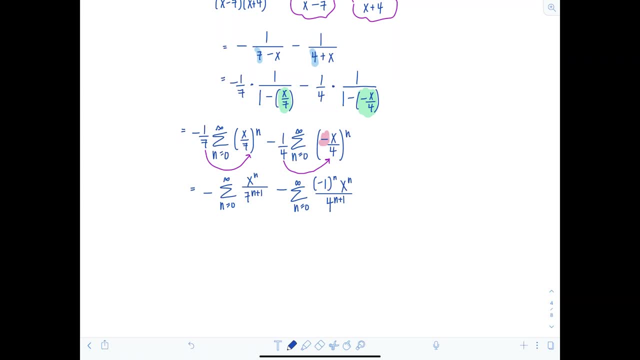 0 go up to infinity and there's a negative on each. so what I can do is factor that on the outside so I can write this as negative: sum n equals 0 to infinity, 1 over 7 to the n plus 1, and then I'm going to add, now that I took out the negative: 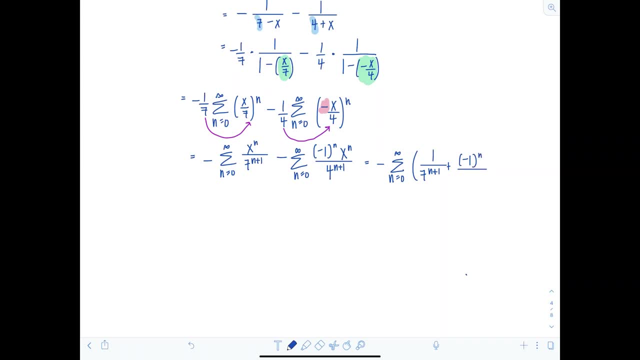 negative, 1 to the n, over 4 to the n plus 1 close parentheses, and then I just have x to the n sitting outside. So notice, basically what happened was I factored out this x to the n from both of the series here. it is. the negative also got factored out here, and then I can write them. 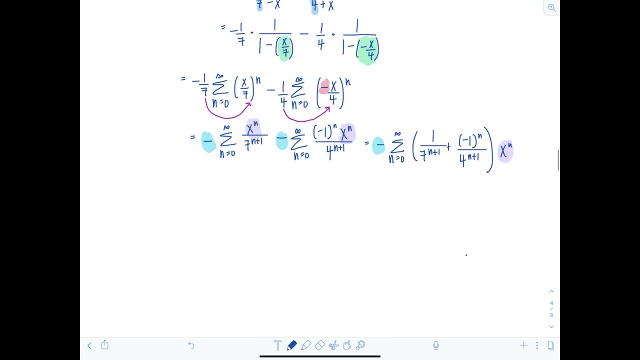 together with one sigma. So just to recap, this means that 11 over x squared minus 3x minus 28, our original f of x is equal to the opposite of the sum. n equals 0 to infinity. I have 1 over 7 to the n, plus 1, plus negative 1 to the n over 4 to the n, plus 1 times x to the n. 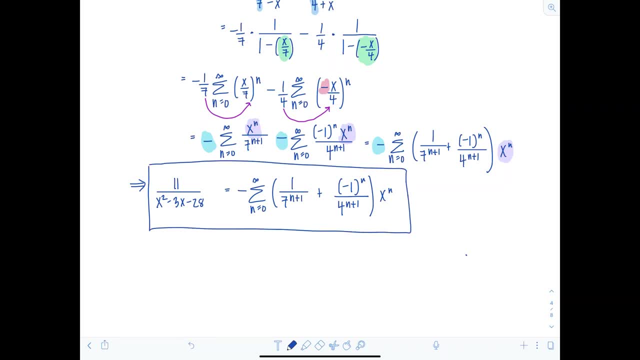 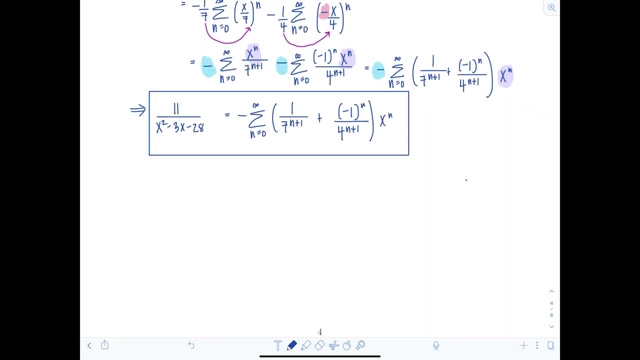 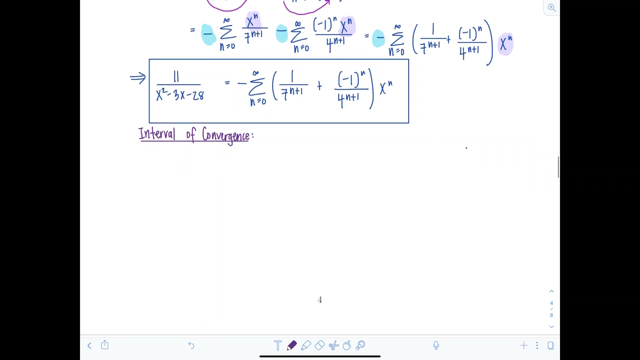 Okay, Now we need to find the interval of convergence. So I have to work with each of these power series that comprise f of x separately. So for the interval of convergence, let's begin with the first sum. So for the sum n equals 0 to infinity. 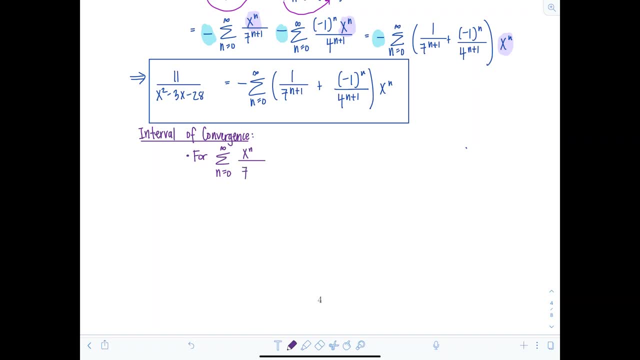 I'm just going to look at x to the n over 7 to the n plus 1. the negative on the outside won't impact anything here, so I need to require that the absolute value of r, which is the absolute value of x over 7.